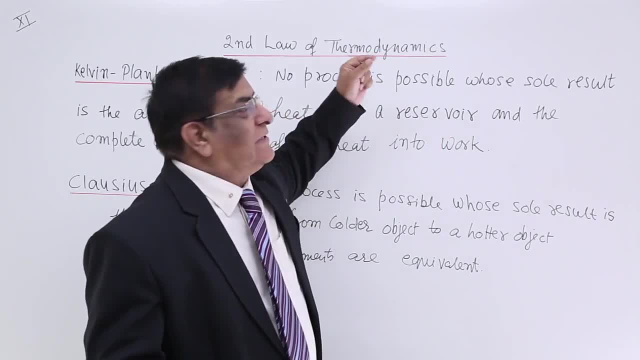 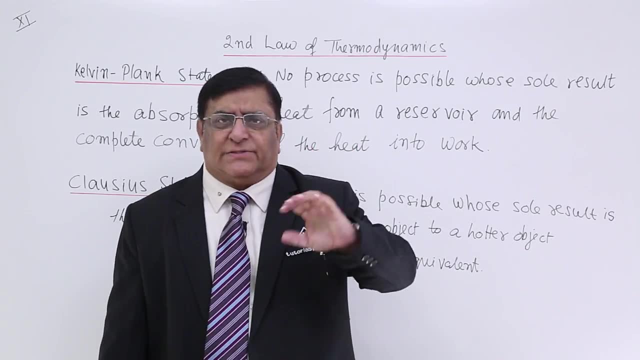 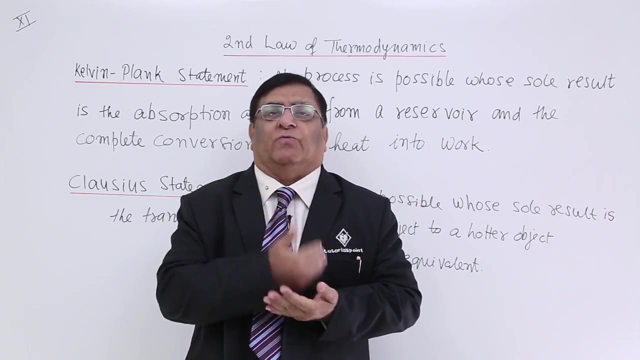 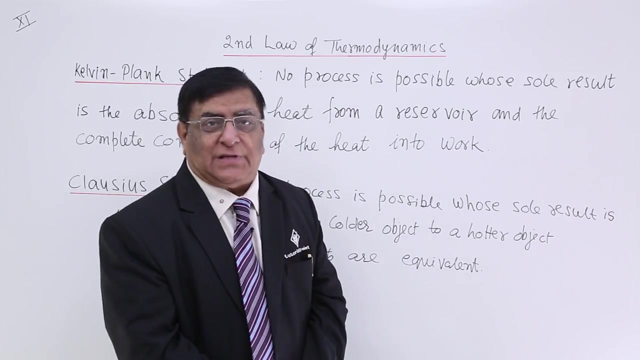 So let us see here. The second law is stated by many scientists in their own language: All means to the same thing, but everyone has understood by his own method and expressed in his own words. So we have taken two very important and prominent scientists, physicists, and we are quoting their words to tell the second law. 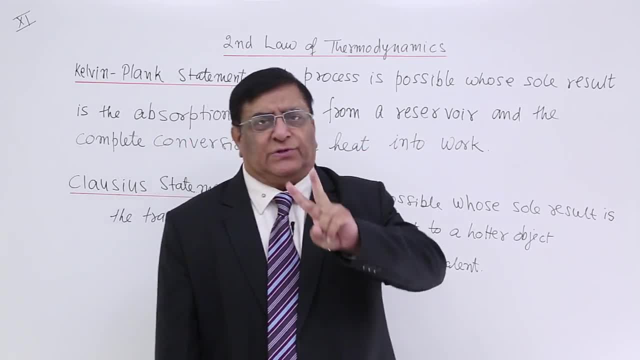 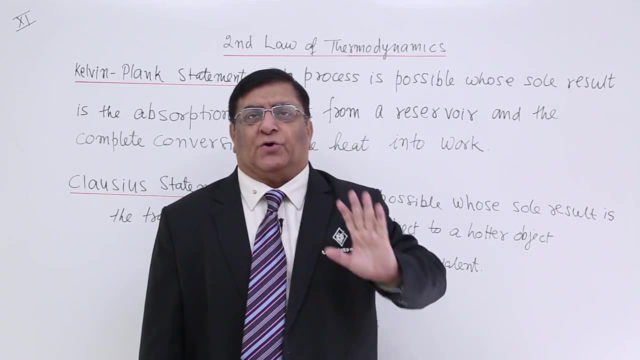 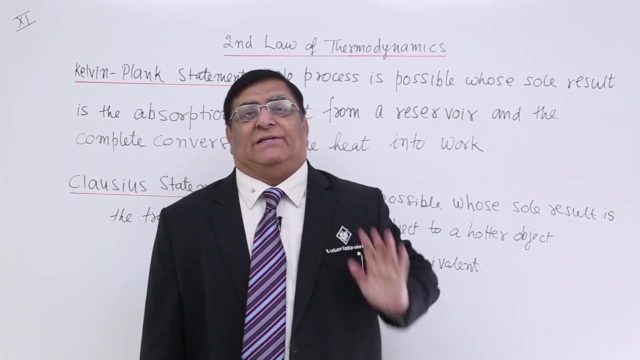 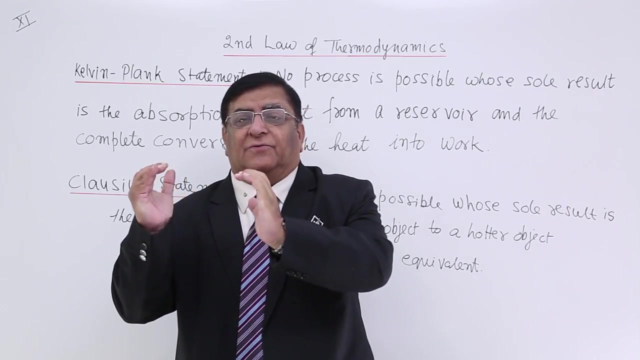 The second law simply says two things: that the efficiency of a Carnot cycle, the efficiency of a process. the efficiency can never be 1, can never be 100% of any machine. If efficiency is 100%, then what will happen? All the heat taken from the source Q1 will be completely converted into work done. 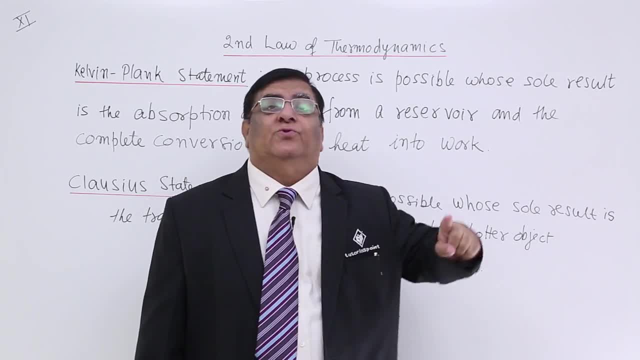 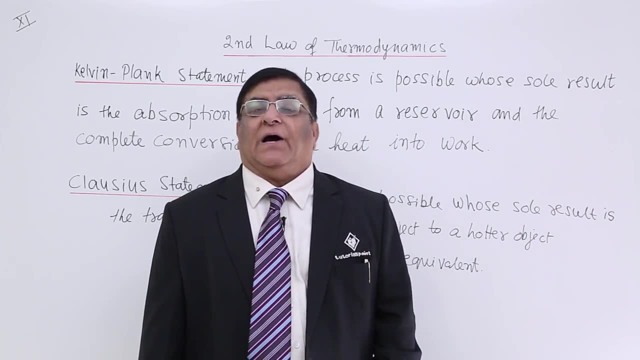 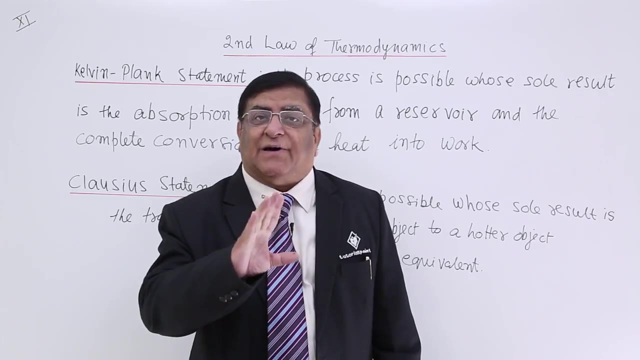 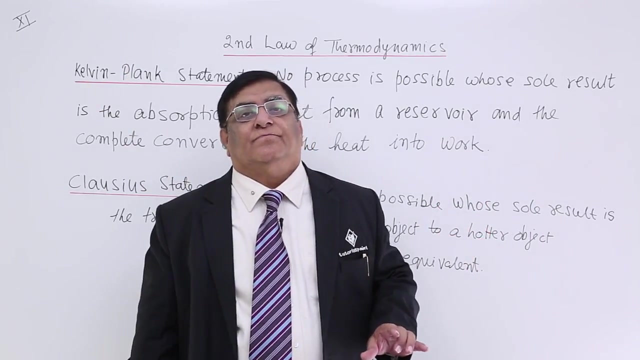 And there is no heat rejected out as Q2 to the sink. So we are not making the flow. That's why it's not possible. This is second law. Other thing: it says that unless we apply a pump, unless then otherwise, there is no way to send the heat from sink to source. So that also cannot be done. 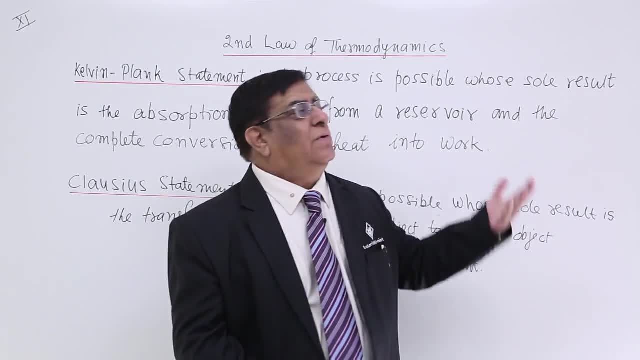 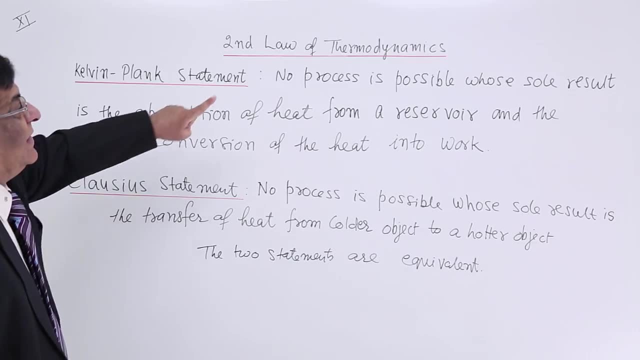 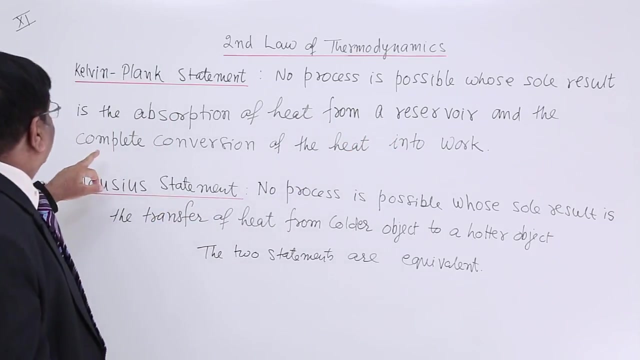 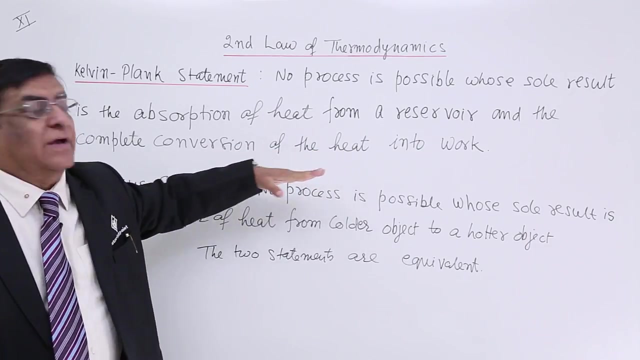 This is second law, So see here how it is given Kelvin and Planck together, they make this statement: No process is possible whose sole result is absorption at heat from a reservoir and the complete conversion of heat into work. Complete conversion of heat into work. efficiency 1, not possible. 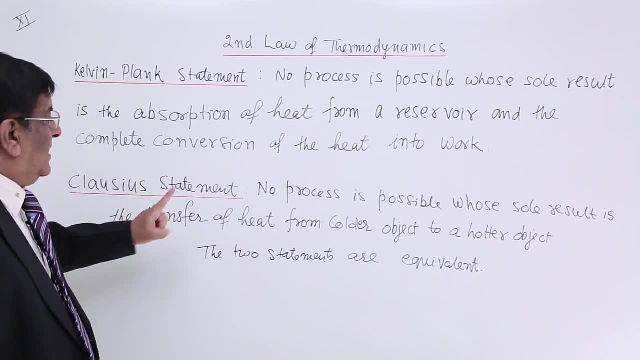 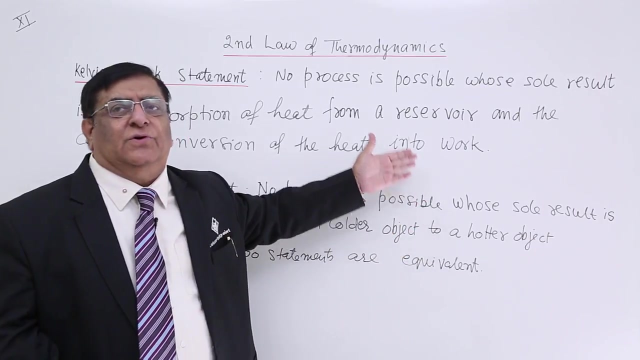 This is second law. The other one says that is by Clausius. No process is possible whose sole result is transfer of heat from colder object to hotter object. That is also one and the same thing, and the two statements are equivalent. Both quote the same thing.